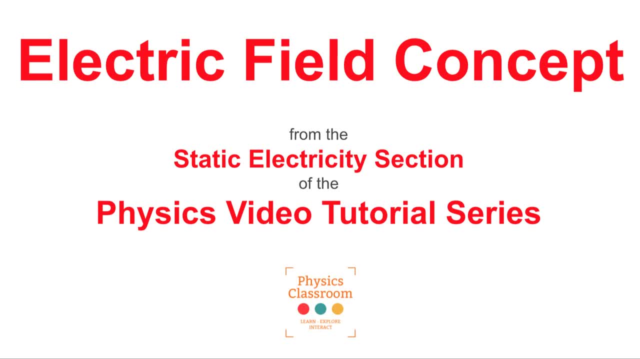 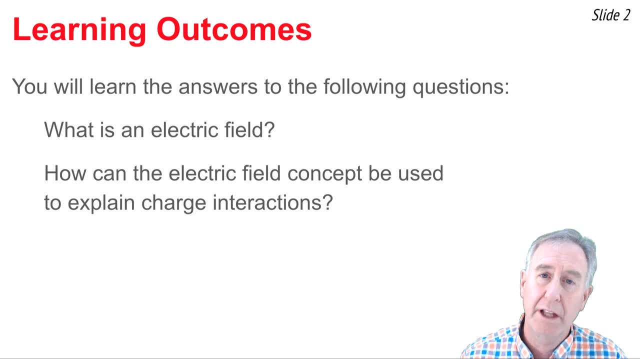 Welcome to the physics classroom's video tutorial on static electricity. The topic of this video is the electric field concept, and here's what we wish to learn today: What exactly is meant by the term electric field, and how can the concept be used to explain charge interactions? Mr H, let's get started. 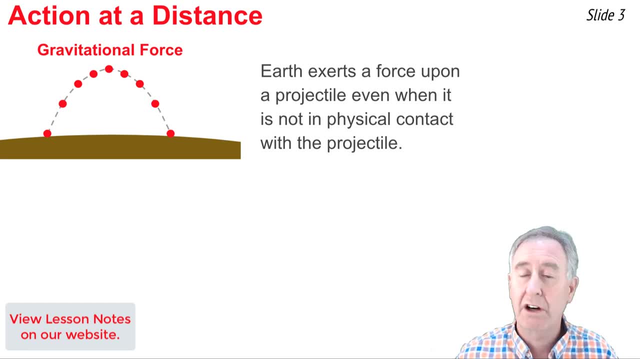 Magnetic forces, gravitational forces and electric forces are all examples of actions that occur at some distance away. Here's what I mean by this. Consider a projectile traveling through the air. As it does, the earth exerts a gravitational force upon it, even though the earth and 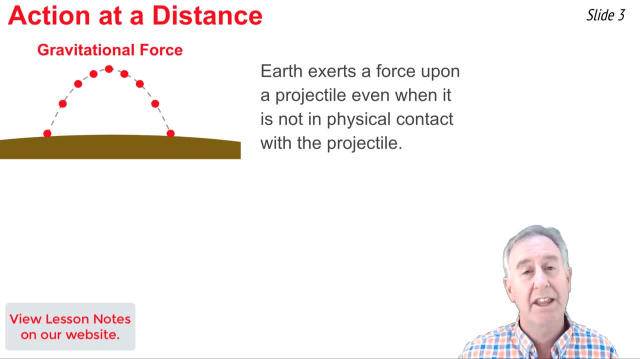 the projectile are not in physical contact with one another. This is an action occurring some distance away. We refer to these types of forces as non-contact forces or field forces. Here's another example: if you have a charged sphere and you bring a balloon nearby, 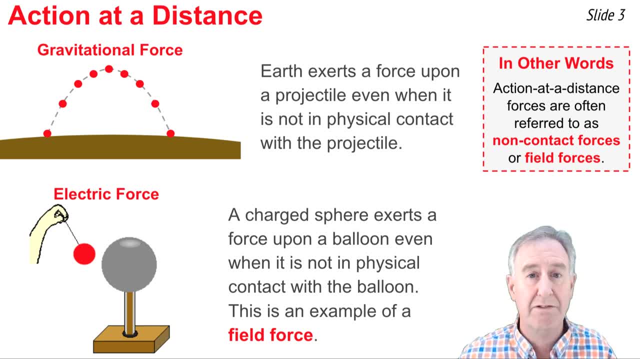 that charge sphere will exert an electric force on the charges of the balloon even though they're not in physical contact with one another. Once more, prend with gravity记 кон 탓" and you bring a balloon nearby. that charged sphere will exert an electric force on the charges of the balloon even though they're not in physical contact with one another. once more. 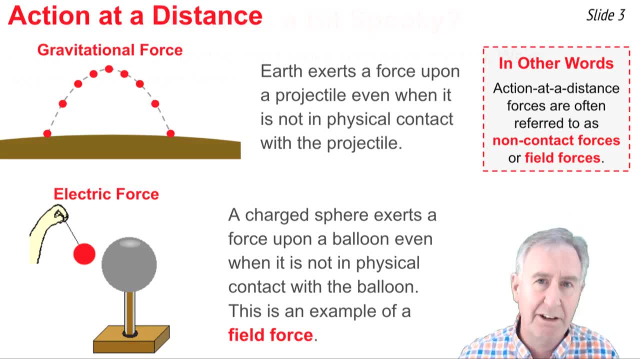 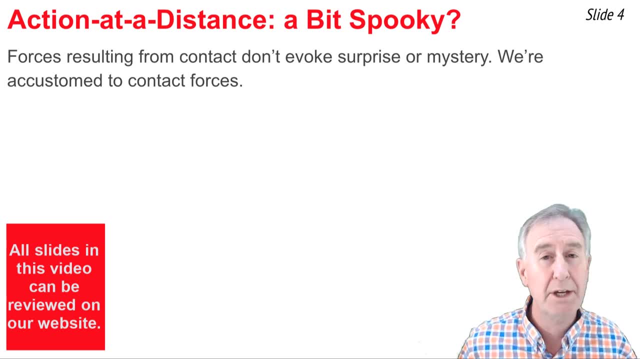 this is an example of an action at a distance, a field force. Forces that result from contact don't necessarily evoke a lot of mystery or surprise because we're accustomed to them, like the force of the seat pushing up on your body, or maybe the force of a baseball in your 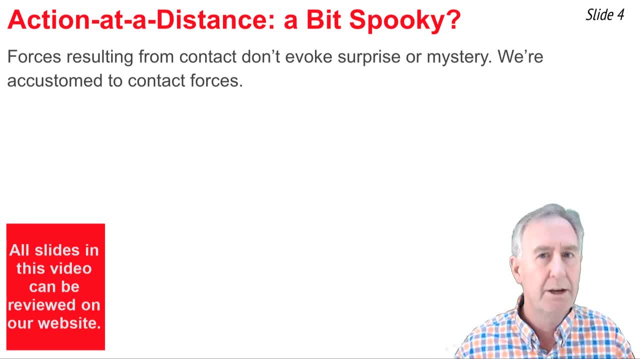 hand as you catch it, or maybe even the force of the linebacker taking down the fullback. in football. These forces are contact forces and they don't typically surprise us. but if you reached out to catch that baseball and while it was still five feet away, it started to slow down and 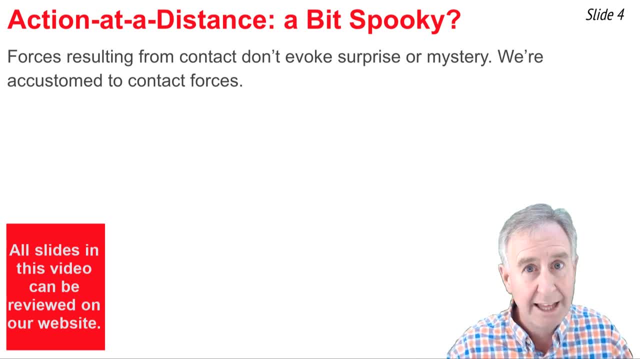 eventually stopped without ever making contact with your hand. that action at a distance would evoke mystery. Or if you were ever watching a football game and, as the linebacker approached the fullback, but before they actually made contact, if the fullback got knocked over backwards. 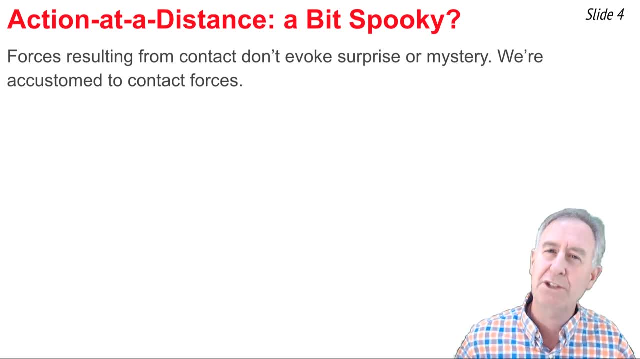 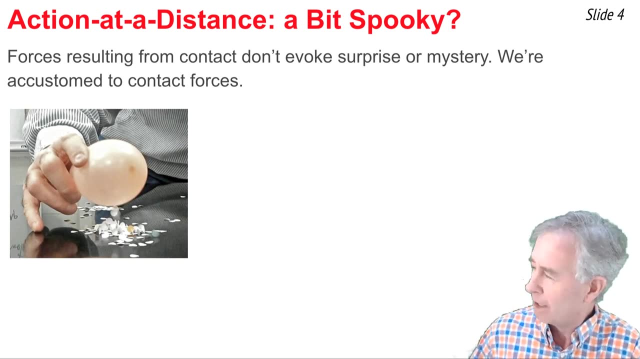 now that would be mystery. In fact, the first time we see certain experiences in physics class that are action at a distance, we kind of think, hmm, that's surprising, Like maybe it's the force of a charged balloon picking up paper bits from. 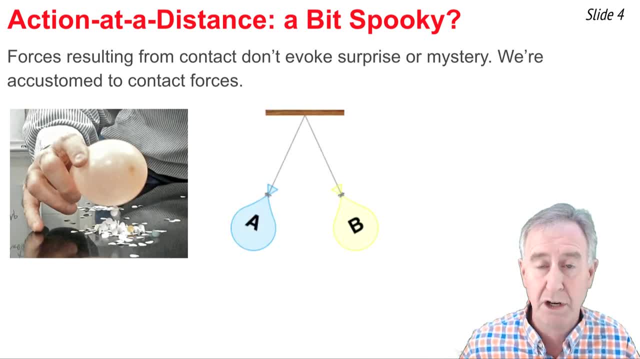 the table. or maybe it's two charged balloons that have light charge hanging from the ceiling and repelling one another. That might evoke mystery. Or maybe if you used an electroscope in your physics class and you brought a both charged balloon nearby it and you notice the 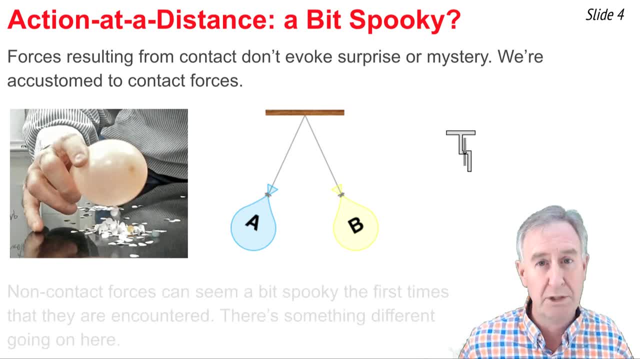 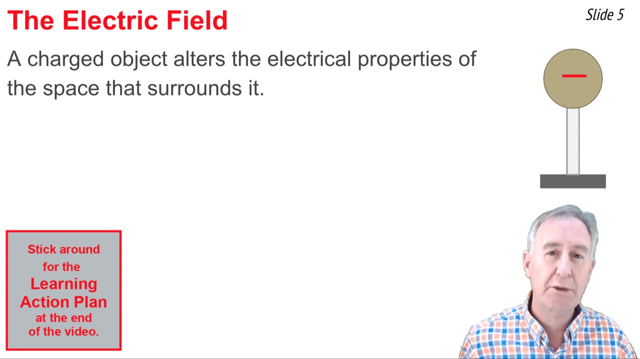 needle of the electroscope begin to move. well, that might evoke mystery. What we're going to do in this video is try to explain action at the distance in all of its mystery, in terms of a concept called the electric field concept. The electric field represents scientists' efforts to explain action at a distance. Here's the logic. 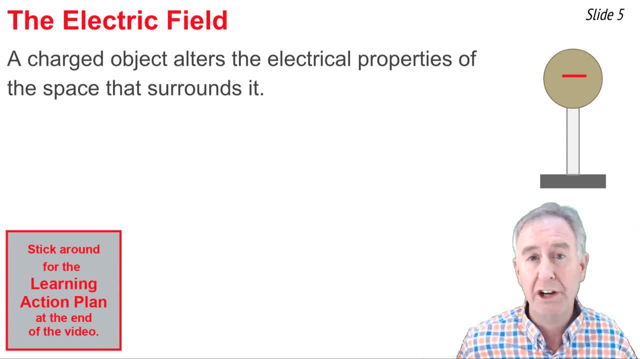 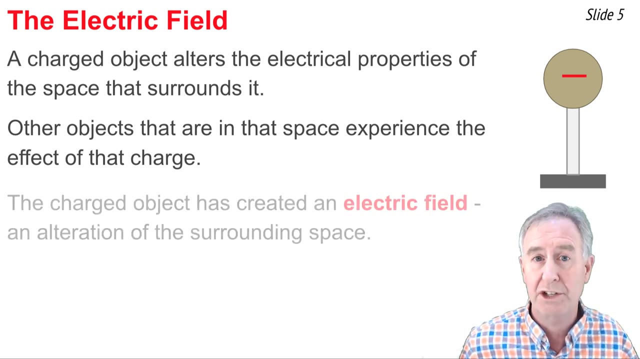 of the idea. A charged object, like a negatively charged sphere, alters the electrical properties of the space that surrounds it such that whenever any other charged object enters into that space, it behaves differently because it feels the effect of the field created by this electric charge. 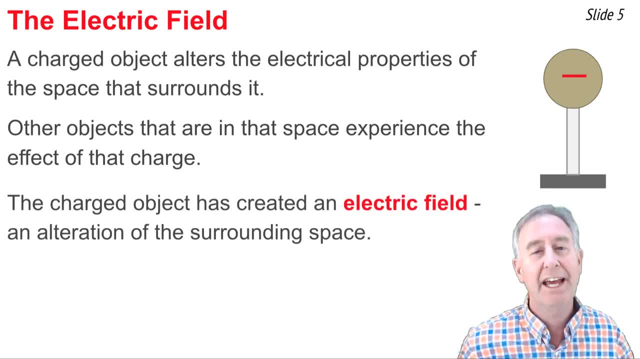 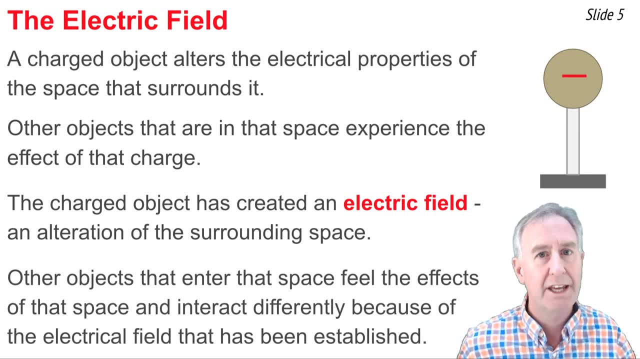 We like to say that the electric field is the agent that creates energy. so if we see that energy creates electricity, we need to know that the charged object has created an electric field, an alteration of the surrounding space, And when other objects enter into that space, it interacts with the 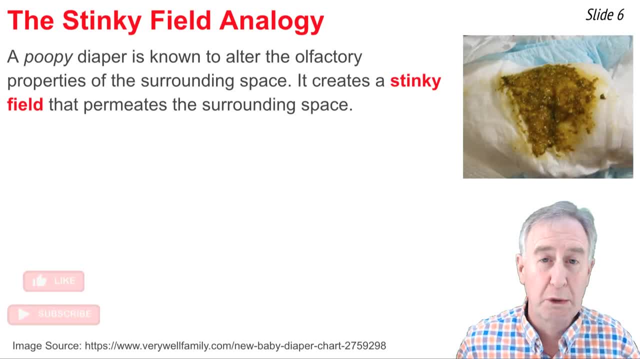 space differently because of the presence of an electric field established by that charged object. A rather crude but useful analogy involves the stinky field created by a soiledor poopy diaper. A poopy diaper is known to alter the olfactory properties of the space that surrounds this electric field. 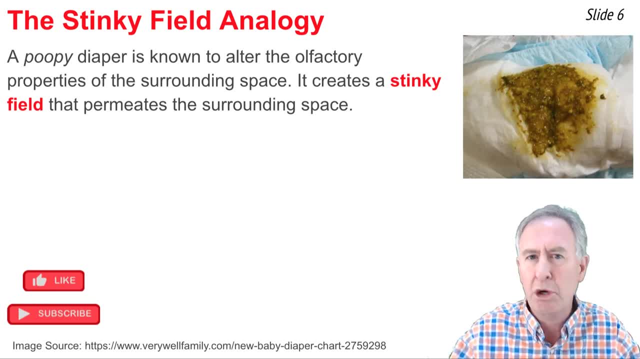 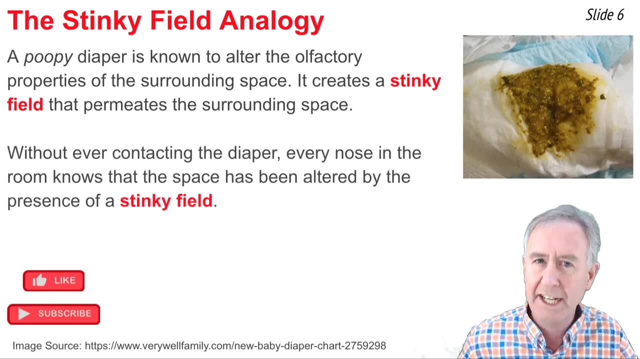 that surrounds it. It creates a stinky field that permeates outward to the surrounding space And every nose in the room, without making physical contact with that diaper, knows that it's in the presence of a stinky field, because it detects something different about the space. 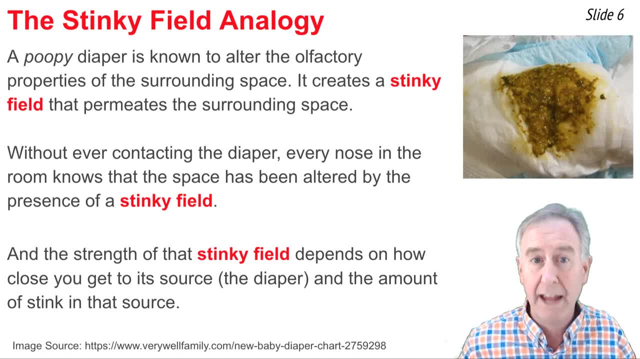 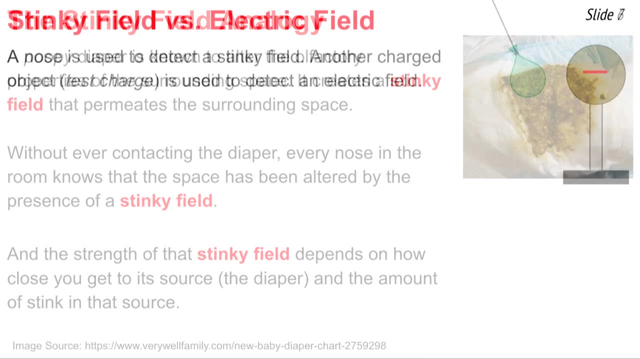 And the strength of that stinky field depends on two main factors: how close your detector gets to the source of stink and how much stink is in that source. We're gonna talk more about what the stinky field teaches us about the electric field. 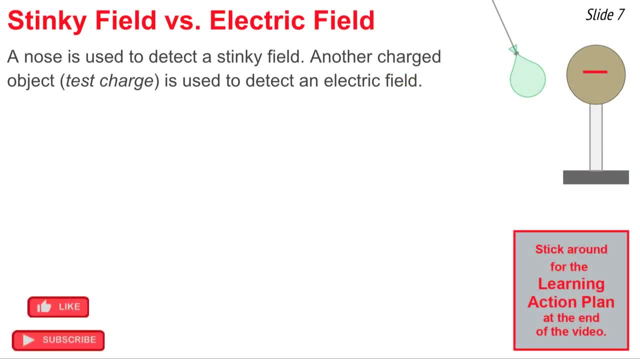 The stinky field is a great analogy for understanding the electric field, And here's why: First, it takes a detector to detect this field. In the case of a stinky field, the detector is the nose, And in the case of an electric field,